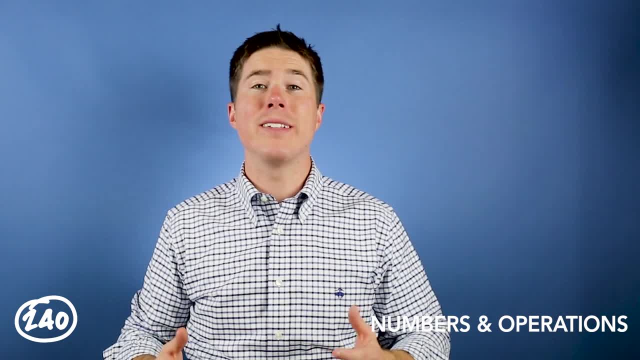 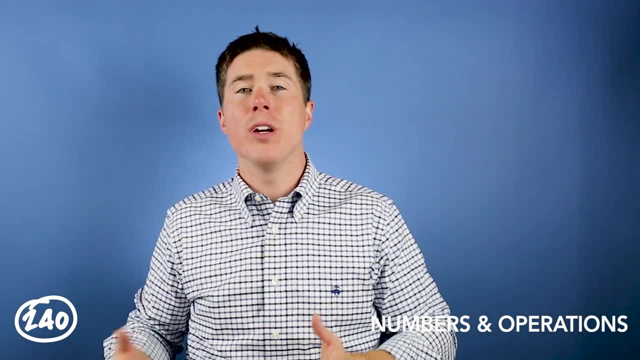 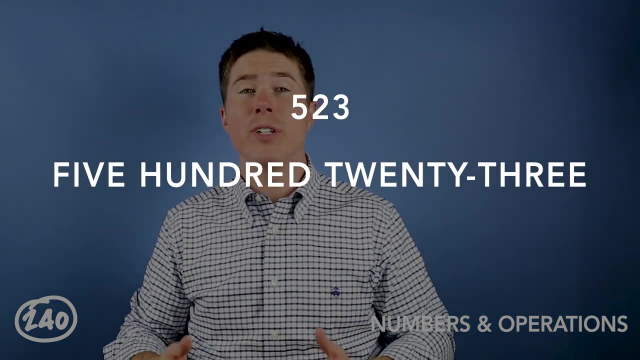 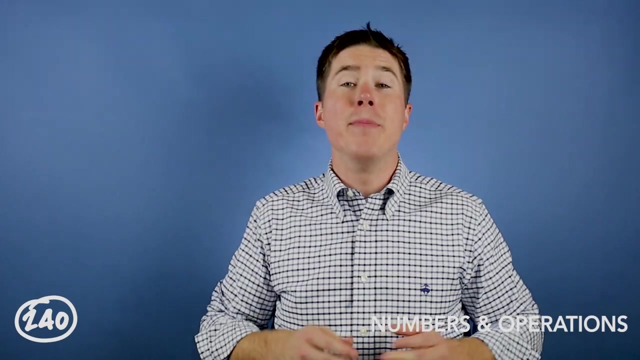 system. you need to know how to write numbers in various ways, including numerals, words and expanded form, for example. here are the various ways to write: the number: 523, you can use the numerals 523. you can use the words 523 or the expanded form 500 plus 20 plus 3.. make sure you understand. 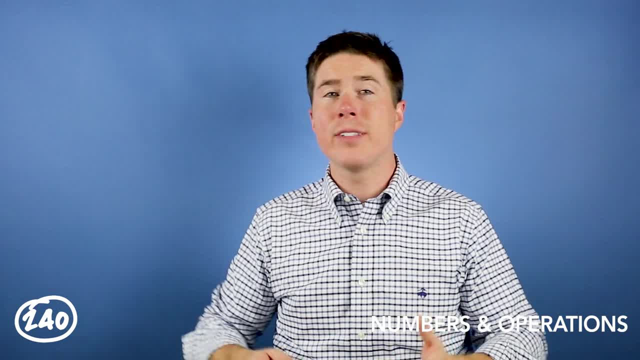 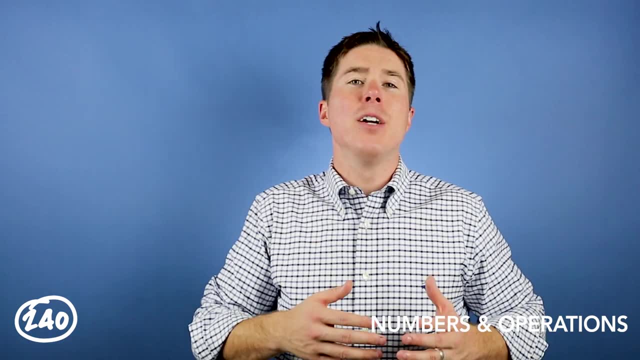 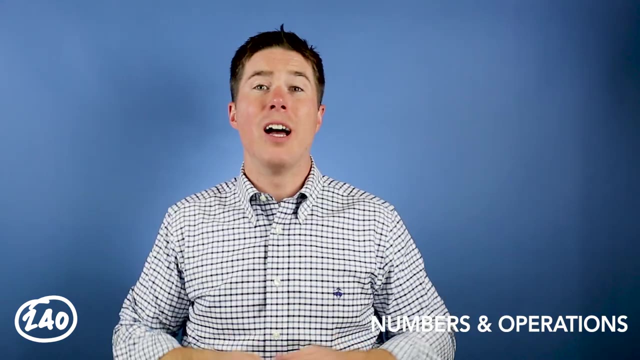 place value, the ones tens, hundreds, etc. both to the left and to the right of the decimal and an exponent. finally, practice rounding numbers to any place value. you'll have to round numbers to the nearest tenths, hundreds and thousands. another big concept to know is operations in rational numbers. a rational number is a number that can be written. 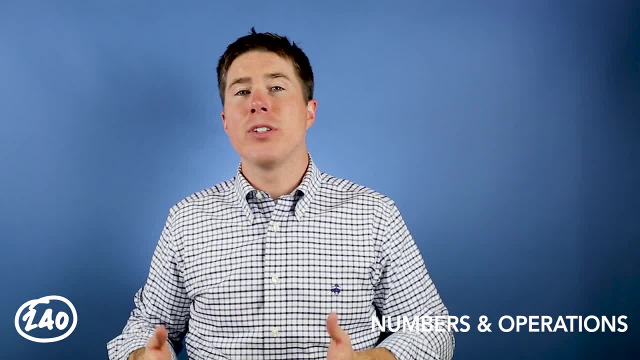 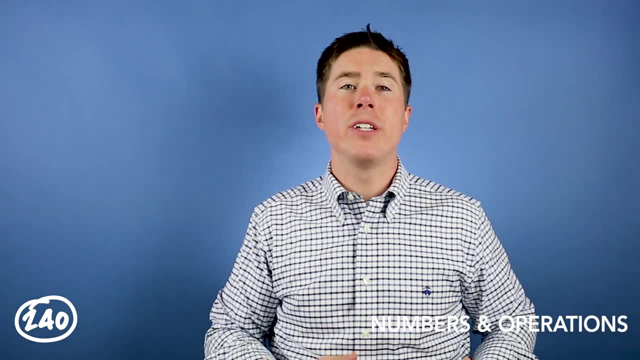 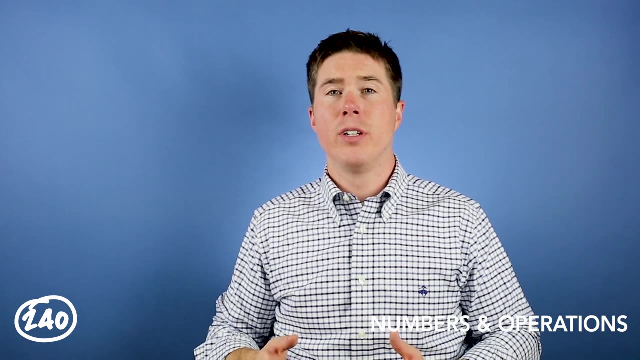 as a fraction or ratio. examples of rational numbers include seven, one point seven, five negative point six and point one one one. you will be presented with multiple step in real world problems where you must conduct operations with rational numbers when using division, be comfortable with remainders and also do lots of practice problems with fractions. 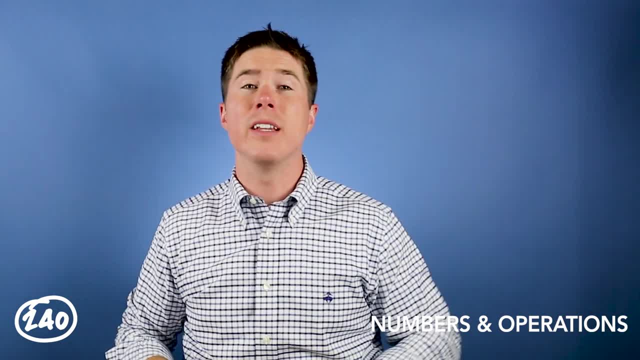 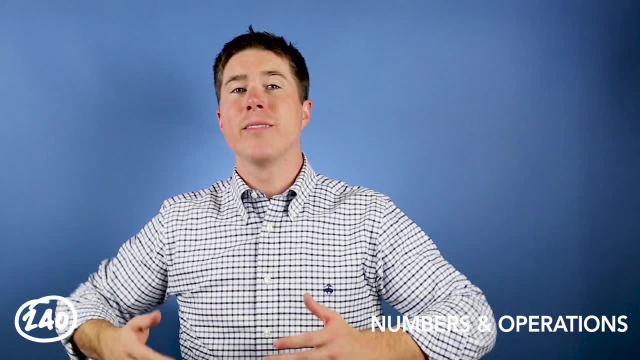 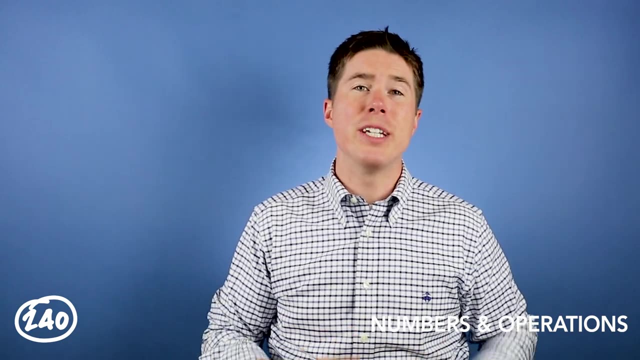 most importantly, you have to know the order of operations- i'll talk about that later in the video- be prepared to represent numbers on a number line- you'll see numbers represented in drawings, models and even arrays- and finally be comfortable with converting between fractions, decimals and percentages. and the last big concept to be familiar with is number theory and reasoning. so 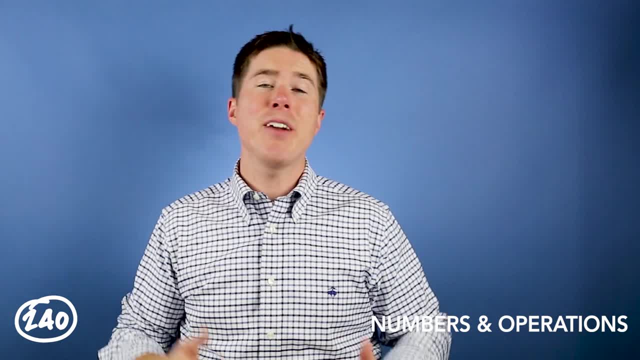 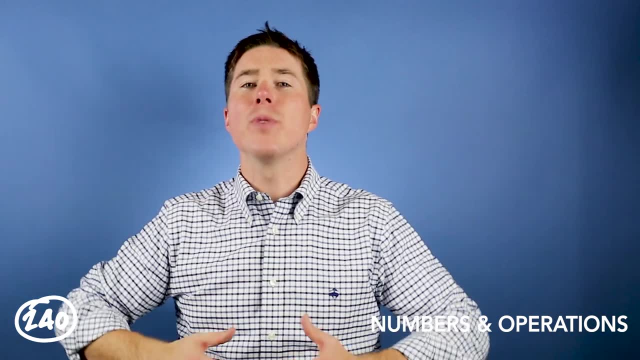 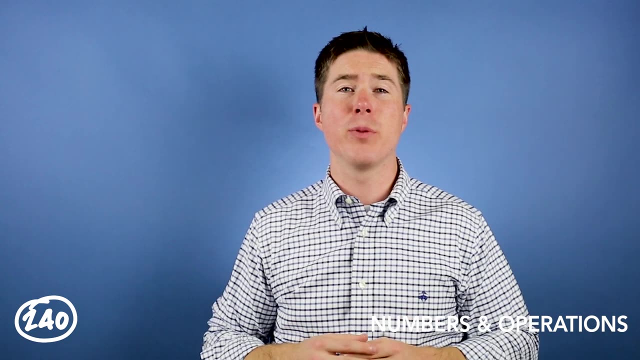 you need to know what prime and composite numbers are and how to find factors and multiples. you also need to be able to reason and use mental math. now, those are just three broad concepts to be familiar with. right now. i'm going to give you three specific concepts to be familiar with because they will most likely appear on the 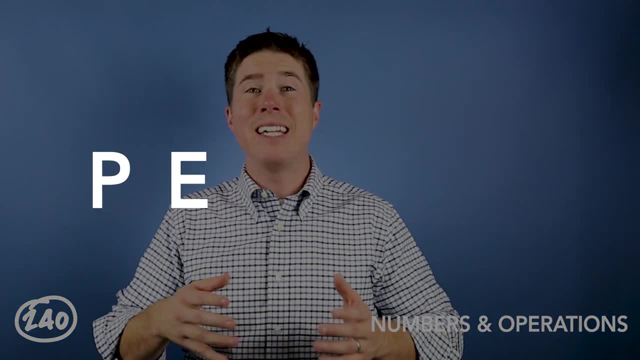 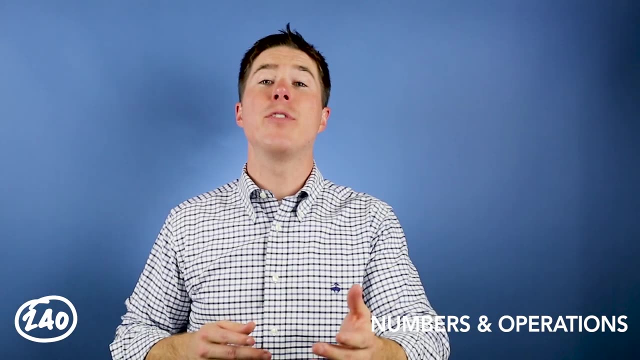 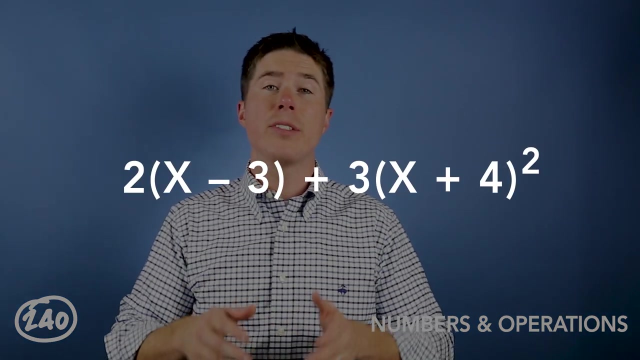 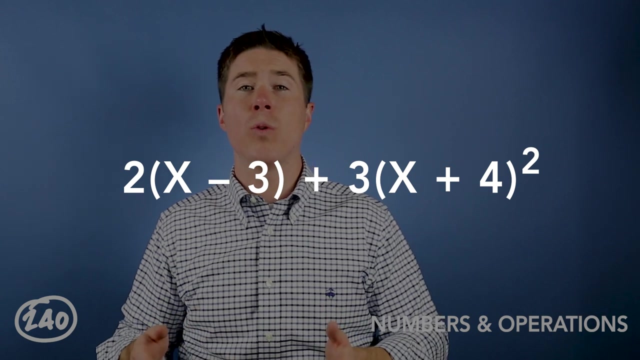 test the order of operations, or pemdos. p e m d a s is simply the process you follow to work through and simplify an equation. let me give you an example. if you have an equation like two parentheses x minus three plus three parentheses x plus four squared, you have to work the problem according to a specific. 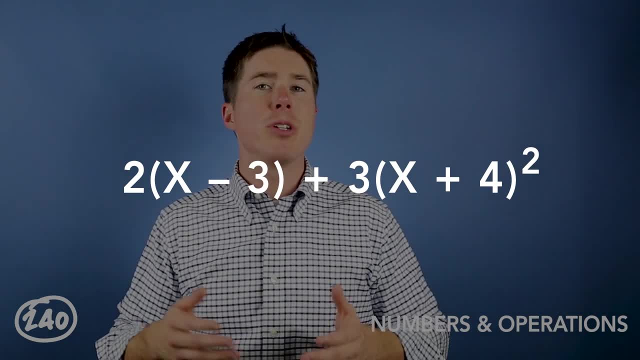 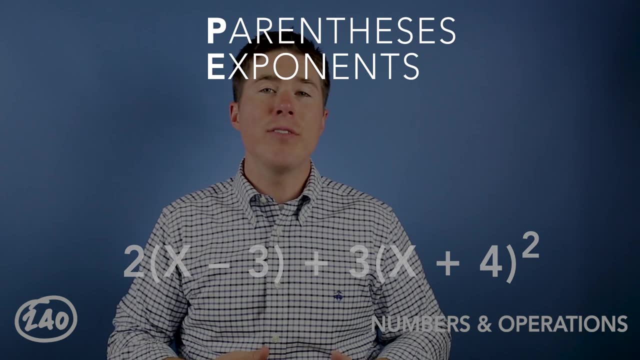 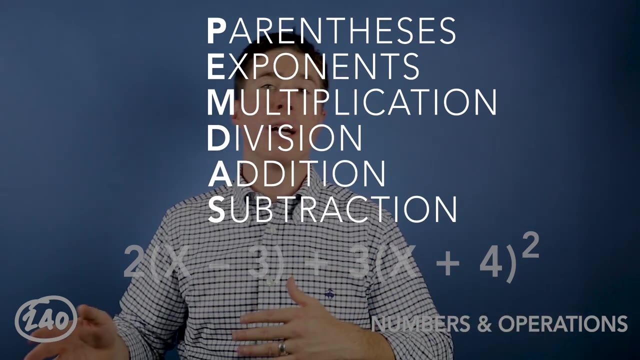 order, the order of operations. in this particular example, you would first solve for the parentheses, then you would solve for the exponents, then, going left to right, you do either multiplication or division and then you would either do addition or subtraction, in the same order left to right. 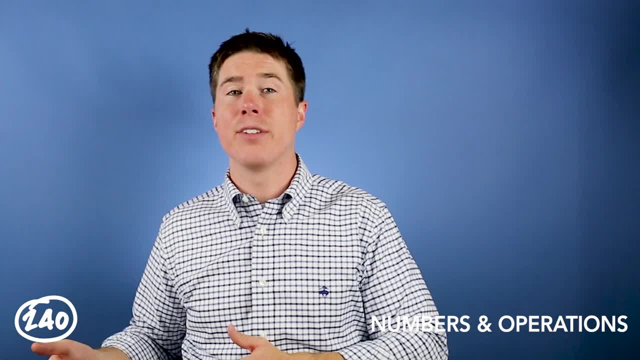 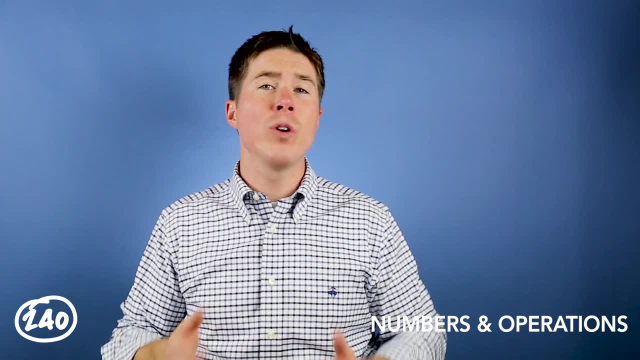 so that's why we group the m and the d and the a and the s together. now, this is incredibly important on the test because you will be required to simplify an equation, so you have to know the order of operations to get that question correct. the next thing you'll see: 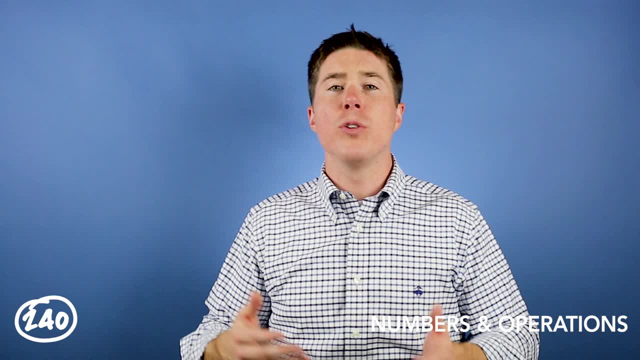 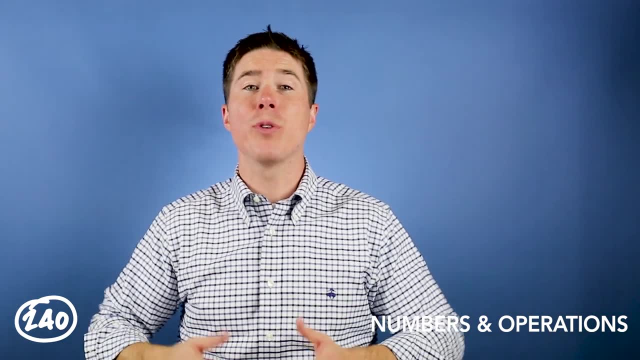 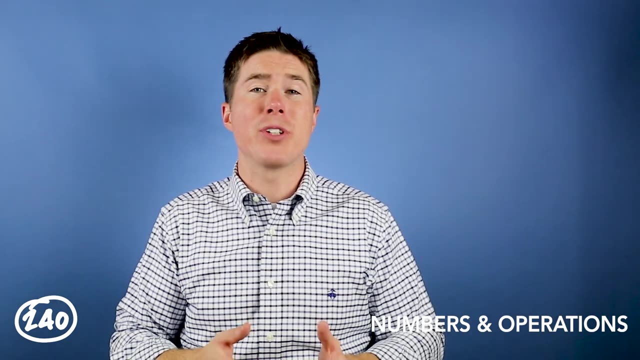 on the exam are word problems. these problems will include all four operations: addition, subtraction, multiplication and division. now my biggest tip to help you with this is to simply work through a lot of authentic practice questions, specifically word problems in mathematics. now, while these questions aren't going to be the most complex, it does take a lot of practice to 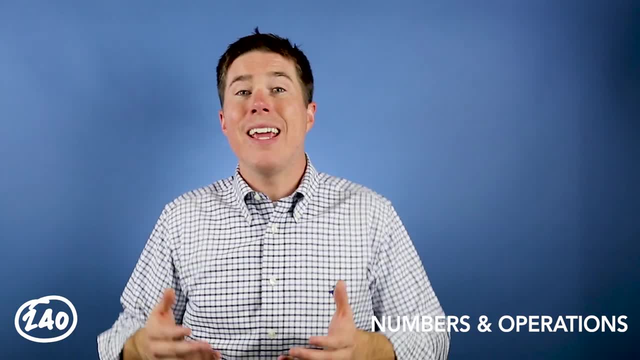 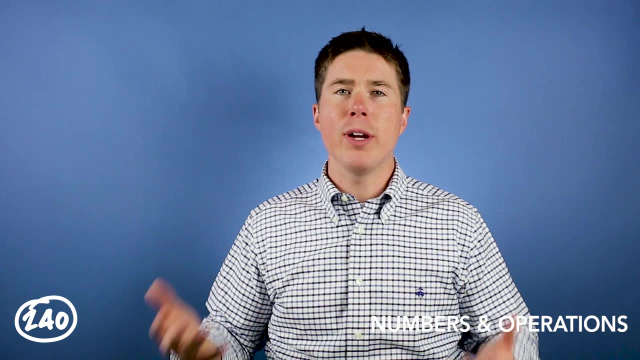 learn how to read a question prompt, understand the question and then solve the problem, and really it's just one of those things that you have to practice, practice, practice. so find a great resource of authentic practice questions that you can use. i'd personally recommend a 240 tutoring. 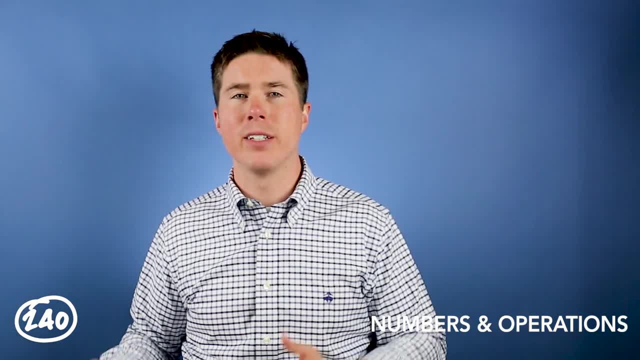 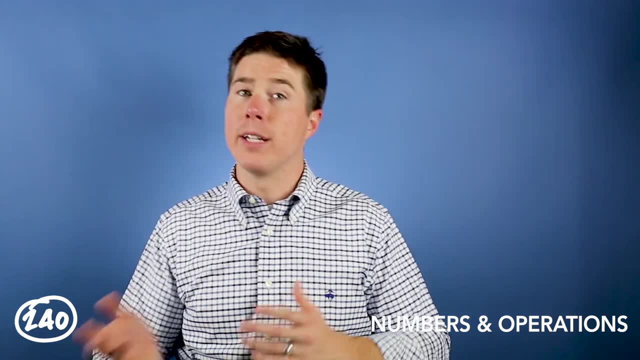 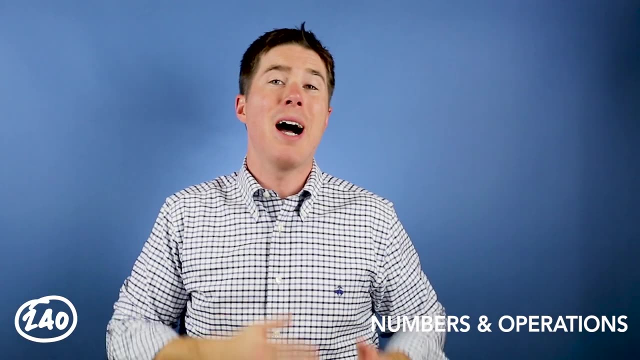 study guide, and the last specific concept is prime and composite numbers. a prime number is a whole number that cannot be made by multiplying other whole numbers together. besides the number one and itself, example of prime numbers include two, three, five, seven and a half and eleven, and there are many, many more now. a composite number is a whole number that can be. 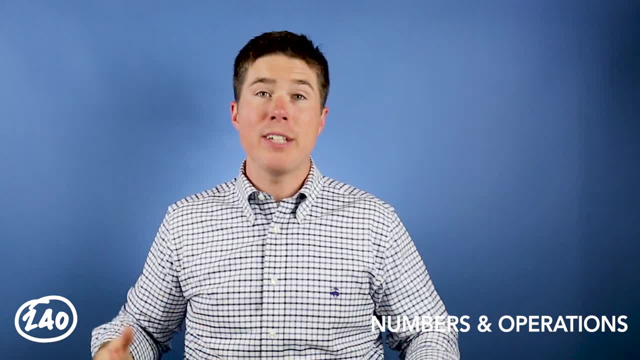 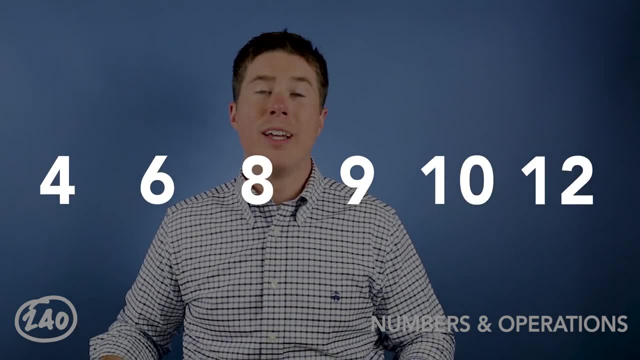 made by multiplying two other whole numbers together besides one in itself. examples of composite numbers include four, six, eight, nine, ten, twelve, and there are many, many more. if all this seems like a lot, it's because it is. there's a lot to know on the exam and if you want to pass, 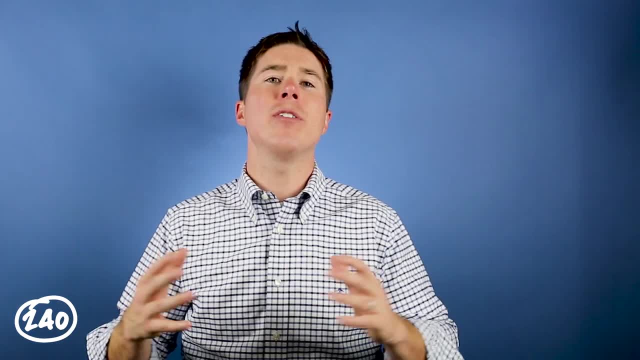 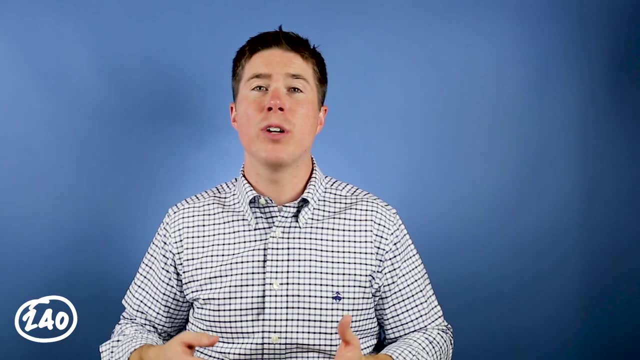 it. you have to study now. the good news is that 240 tutoring already has done all the hard work- figuring out how to study and how to create the best one in a row, and you'll be able to do it in a very short time. so let's get started. 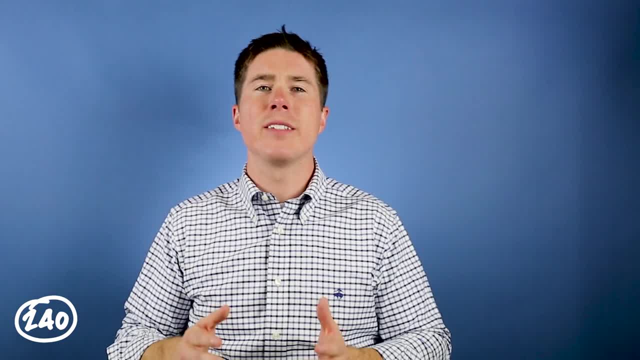 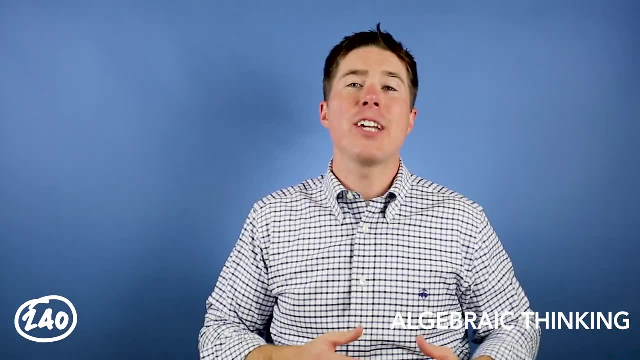 so what you're going to want to do is to make sure that the questions are easy to understand after you have two of these two materials to study, and creating authentic questions to practice the test- oh, and the test is really expensive. so do yourself a favor and save a bunch of time, and 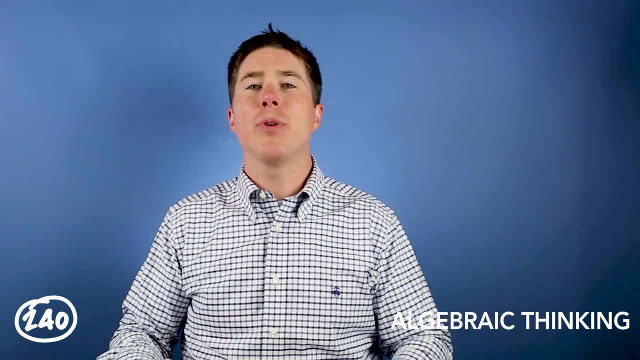 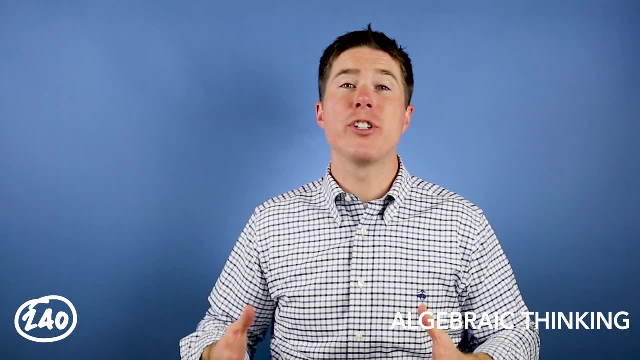 money and simply use a 240 tutoring study guide. let's look at the next section of the exam: algebraic thinking. this section tests your ability to- you guessed it solve algebra problems. algebraic thing questions make up about 30 percent of the mathematics subtest. now there are three big concepts. 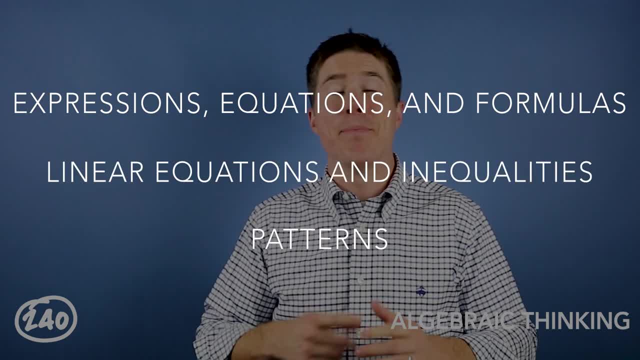 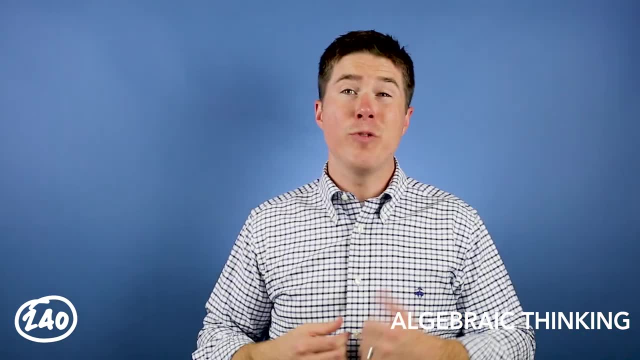 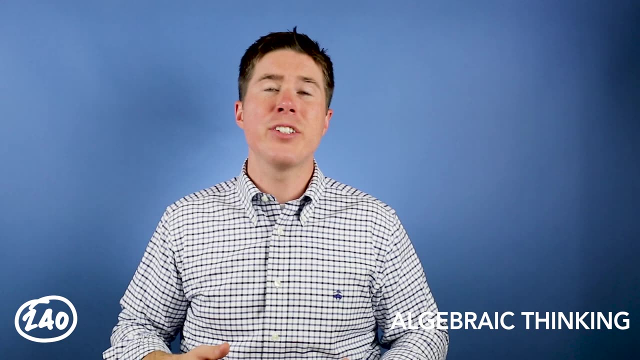 formulas, linear equations and inequalities and patterns. The first big concept you need to know is how to solve expressions and equations and use formulas. First of all, you have to know the difference between an expression and an equation And you will be asked to add and subtract linear equations, to use the distributive 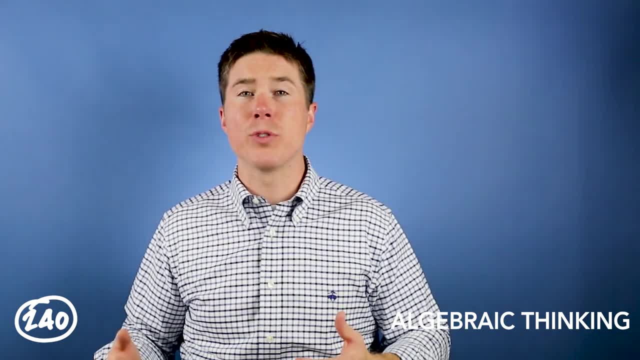 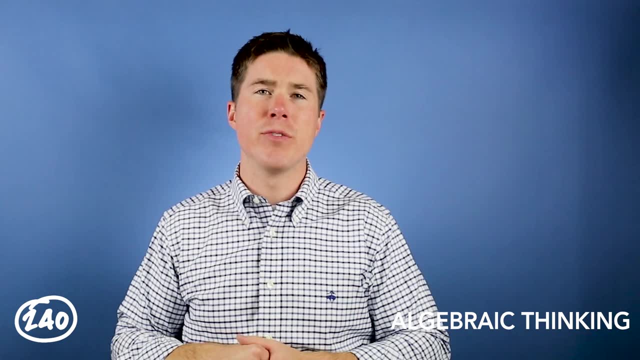 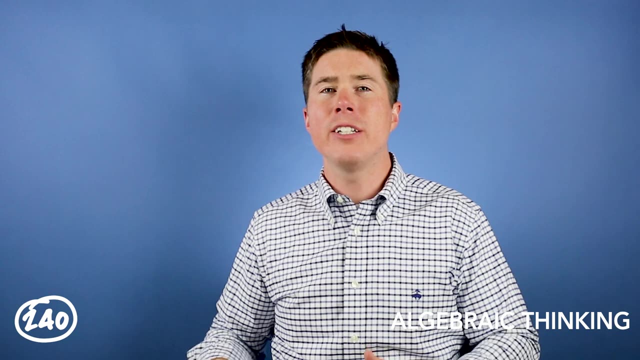 property to solve simple expressions. to use formulas and represent words with equations and expressions. Finally, know the difference between independent and dependent variables and be able to identify each in formulas. The next big concept is linear equations and inequalities. You will definitely be asked to solve linear equations and inequalities, and these will 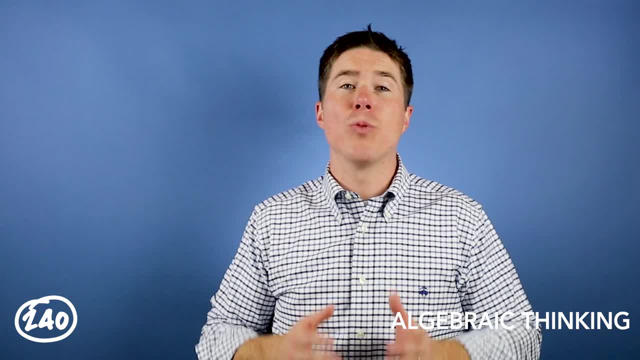 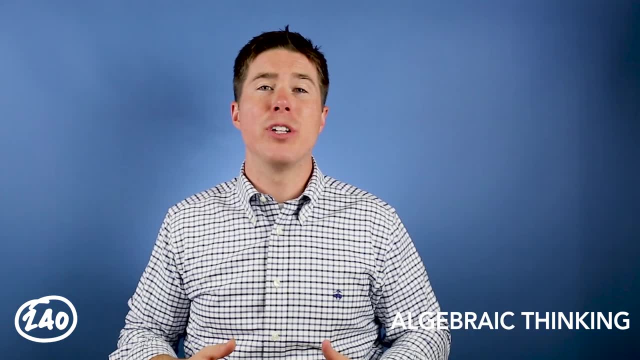 be pretty basic with only one variable, But be ready to graph a solution on a number line and use equations, tables and graphs to solve the problems. Now, the last big concept to know is patterns. You need to be able to identify, extend, describe and multiply. 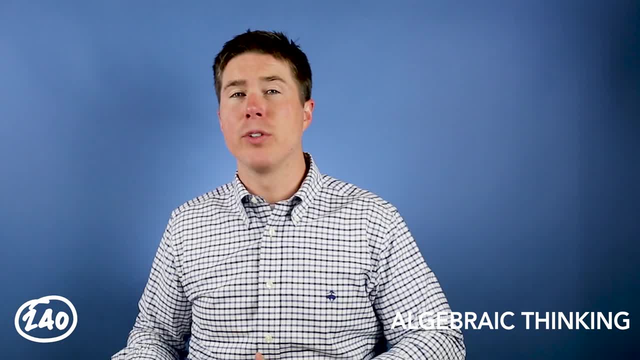 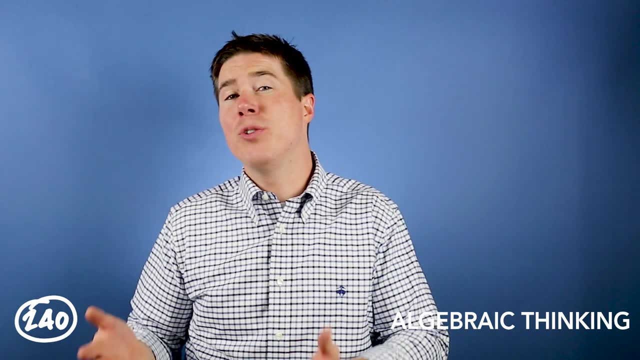 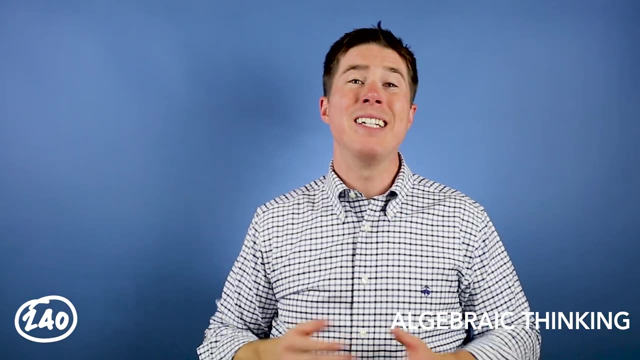 You need to be able to describe and make patterns both with shapes and numbers. On the test you may be asked to have to find a rule for a function table by looking at a set of two numerical patterns. So those are the three broad concepts to be familiar with for the algebraic section. 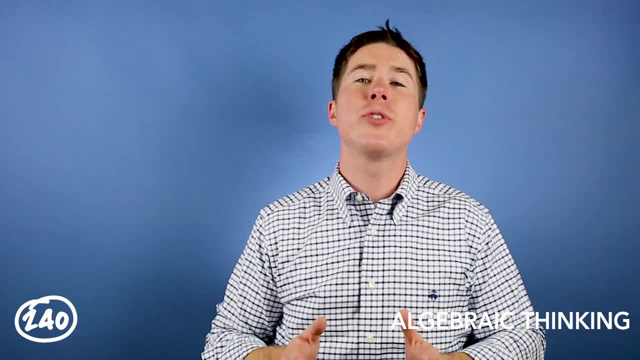 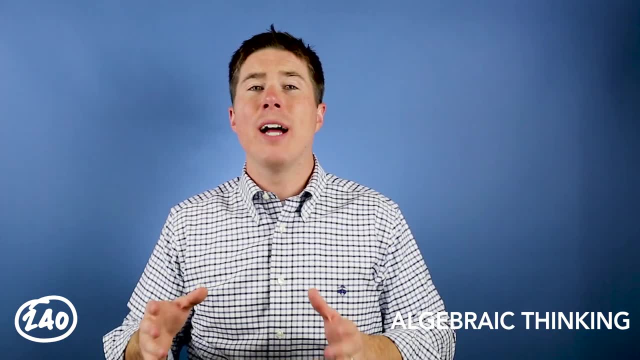 But now I want to talk to you about some specific concepts that are almost guaranteed to come up on the exam. So right now, I'm going to give you three specific concepts that you have to know. You need to know how to solve for x. 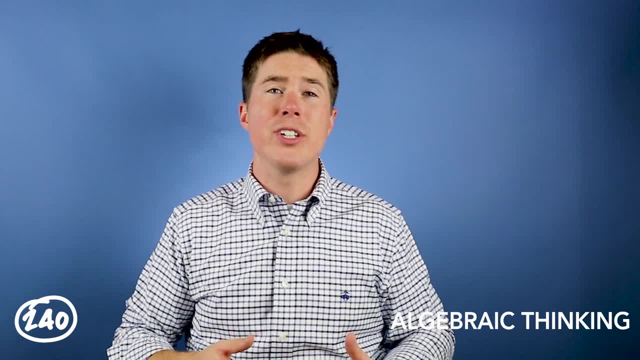 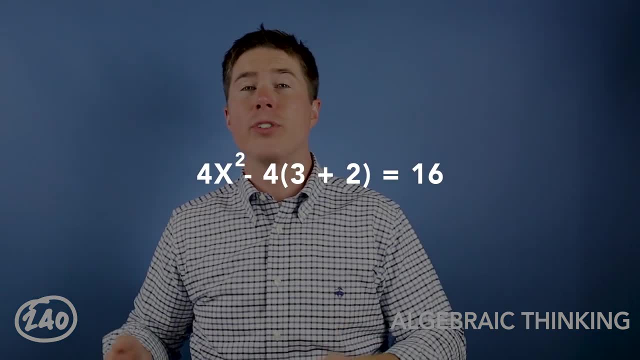 Solving for x is pretty straightforward. The test will give you an equation and then you have to solve for x. So the test will give you something like this: Four x squared minus four parentheses, three plus two equals sixteen, And in this equation we just need to balance the equation for x. so you would simplify it. 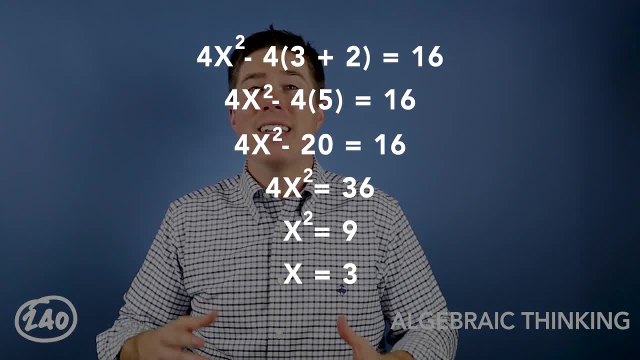 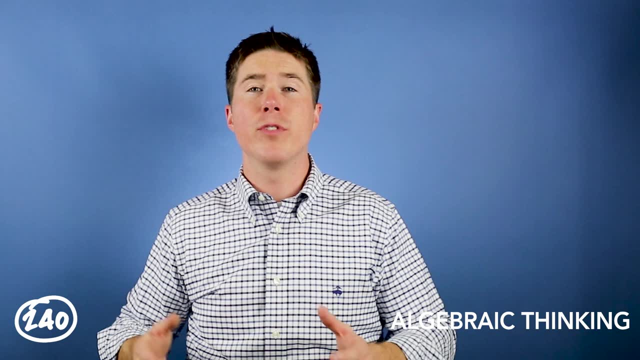 as much as you can balance the equation and you find that x equals three. Now take note, you're more than likely going to be presented with a real-world problem solving for x. So be able to take what you need. Take what you need from the problem, build the equation and solve for x. 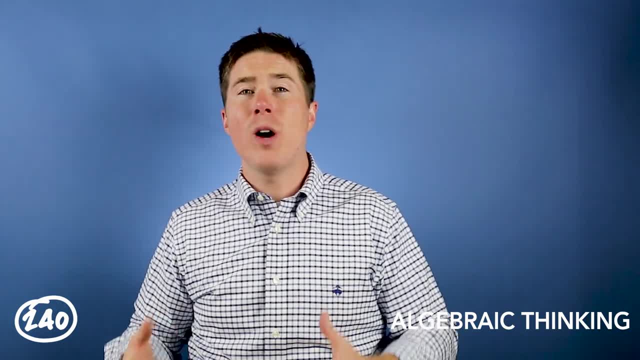 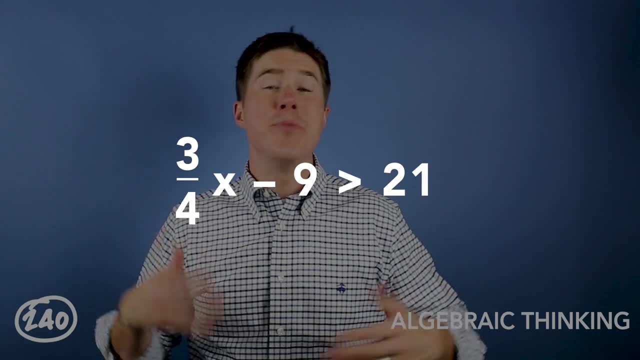 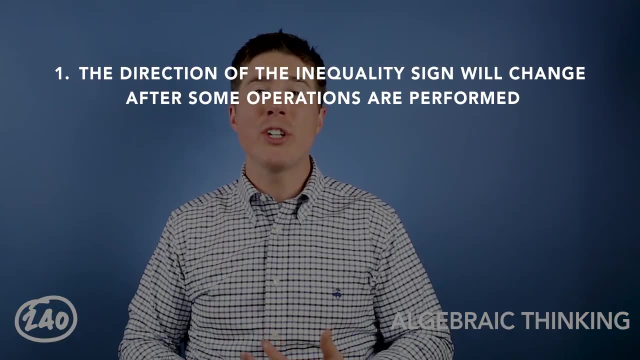 You're also going to have to solve inequalities. Solving inequality statements in one variable, such as three-fourths x minus nine is greater than twenty-one, is much the same like solving an equation. in those addressed above. The only major differences is that one: the direction of the inequality sign will change. 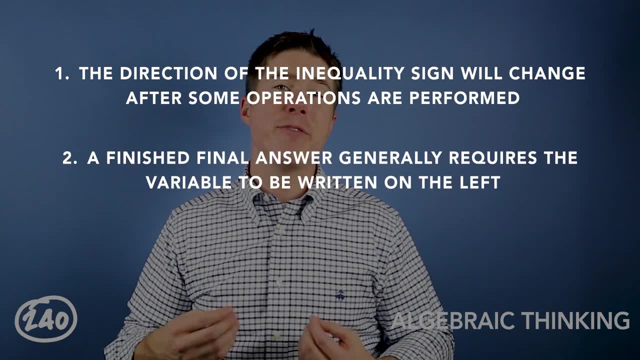 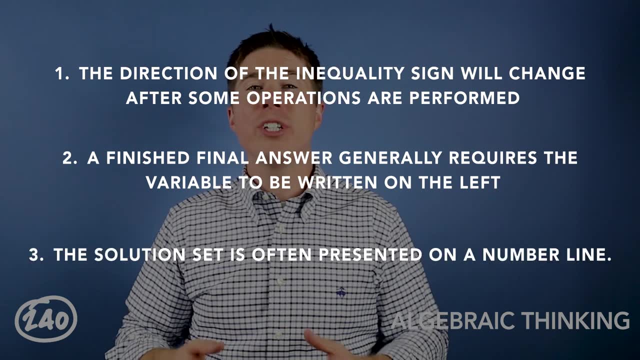 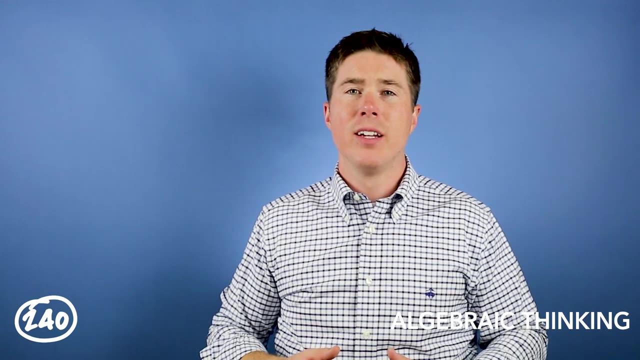 after some operations are performed. And two: a finished final answer generally requires a solution, Generally requires the variable to be written on the left. And three: the solution set is often presented on a number line. Now the next concept is creating an equation from a data set. 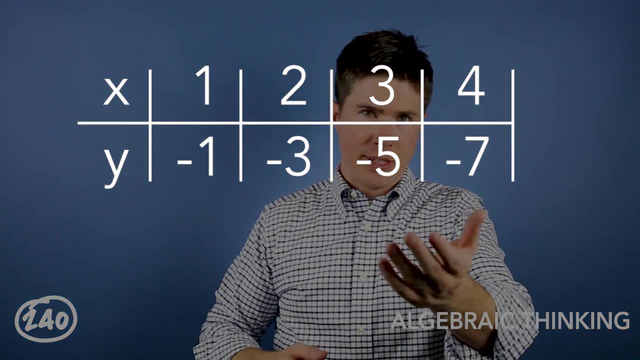 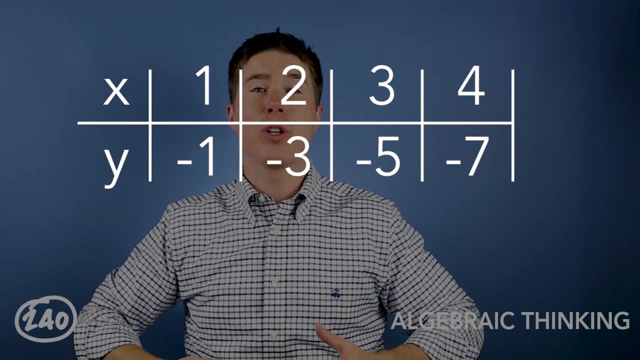 The test will give you a data set that looks something like this on the screen And you're required to create a corresponding equation that matches the data set. For this data set, the corresponding equation is: y equals one minus two x. Now, if you look at the data set, 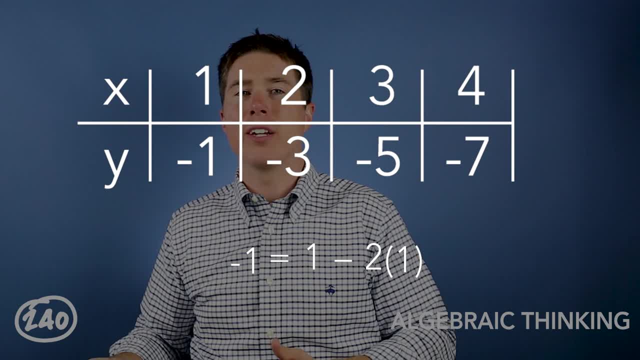 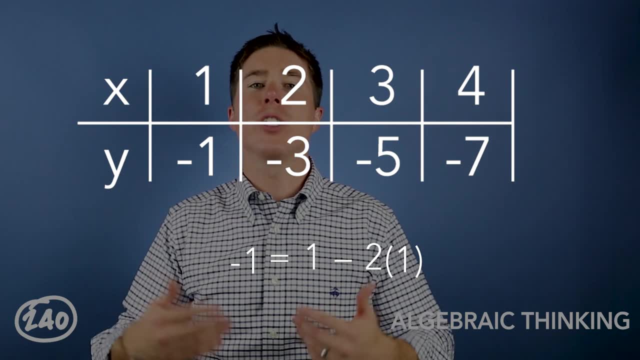 Any time you plug in the x, You get the corresponding y value when you solve the equation. And while this kind of question can seem difficult, it's one of the easier questions to answer if you just work backwards. All you need to do is look at the answer options, plug in the data, set values to each equation. 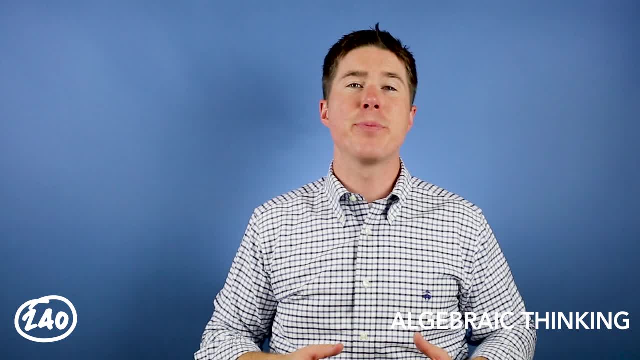 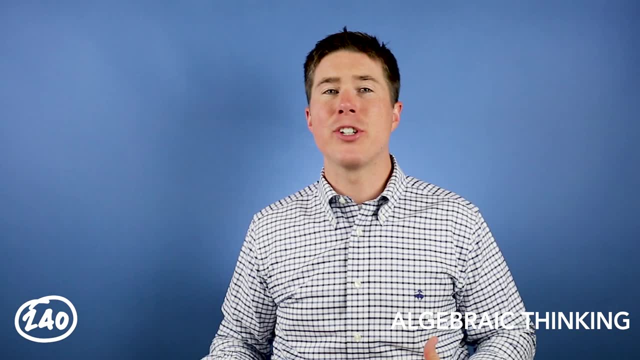 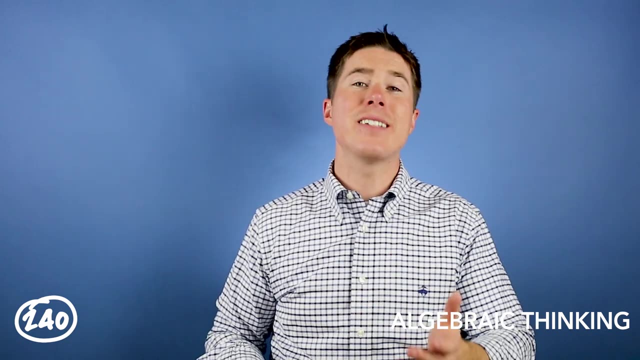 and see if they match. The next concept to know is the difference between equations and expressions, And it's really pretty simple. The main difference between equations and expressions is an equal sign. An equation has one And an expression does not. Look at some examples. 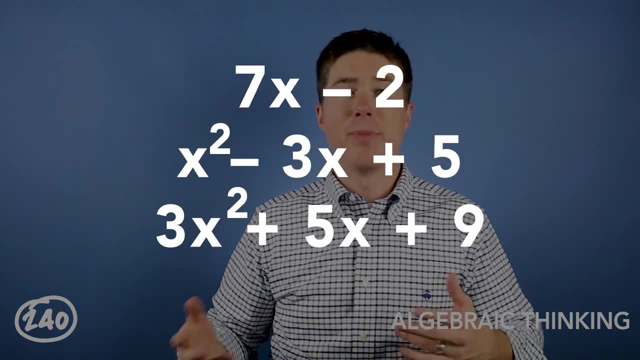 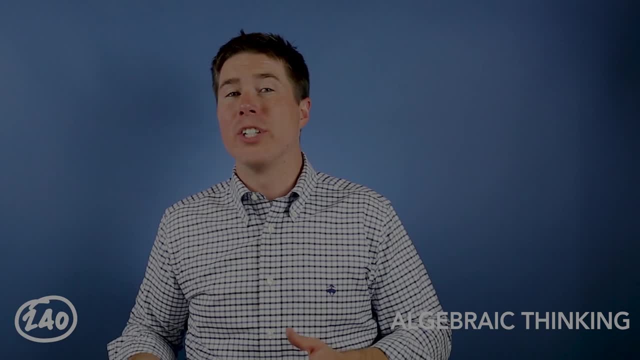 These are some examples of expressions: 7x minus 2.. x squared minus 3x plus 5.. 3x squared plus 5x plus 9.. Now compare that with equations: 8x equals 16.. 2x plus 1 equals 7.. 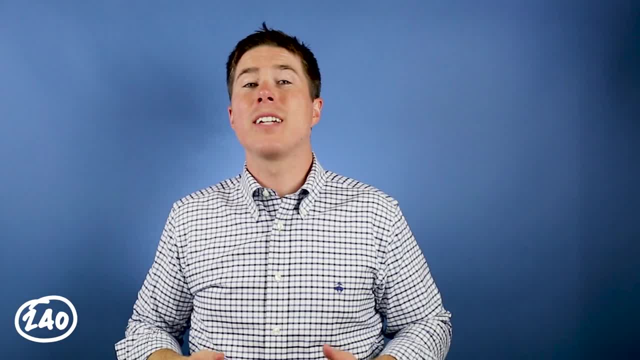 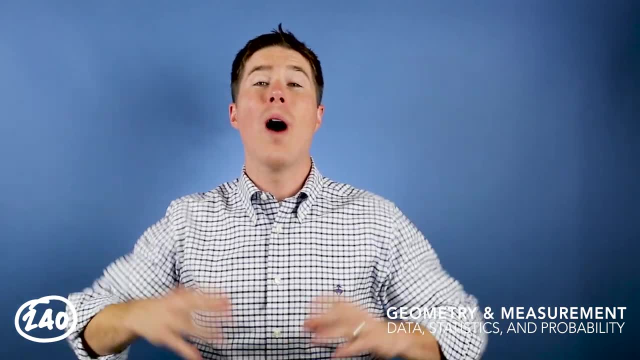 20 minus 7x equals 6x minus 6.. Now let's go ahead and look at the next section: Geometry, measurement, data, statistics and probability. Now this section is really easy. It's really easy. This section is going to test your knowledge on a wide range of math concepts, including 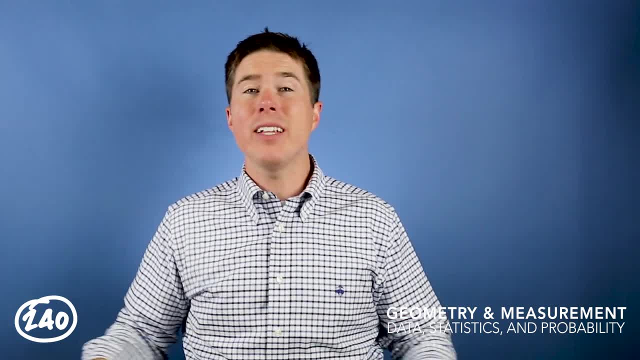 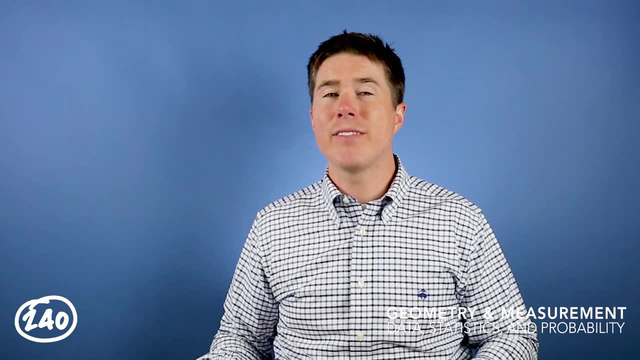 shapes, the coordinate plane, measurement and the likelihood of an event occurring, And this section will make up 30% of the mathematics subtest. There are three big concepts you definitely have to know to get these questions correct: Shapes, measurement, data and probability. 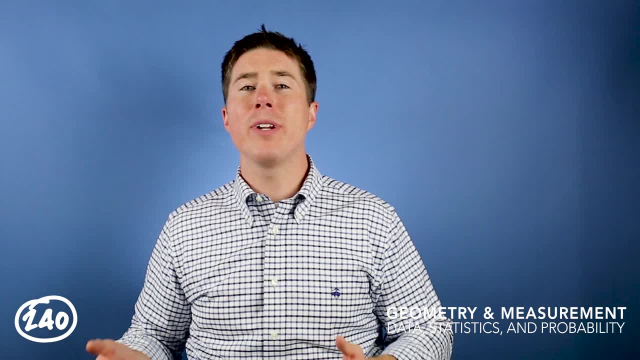 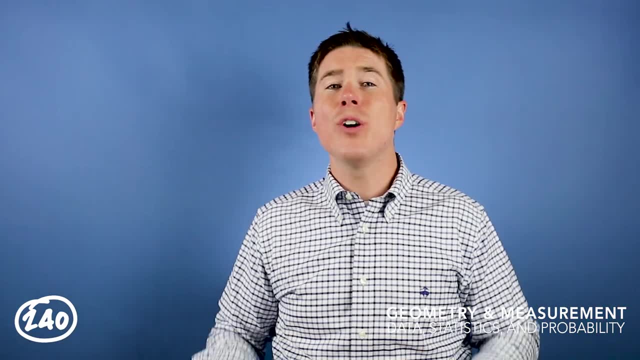 The first big concept you need to know for the test involves one, two and three-dimensional shapes, their properties and how to find the perimeter area, surface area and volume of those shapes. You need to know these terms and how to identify them in shapes like lines, rays, line segments. 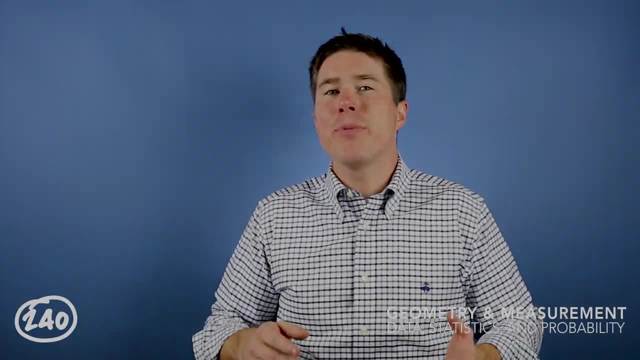 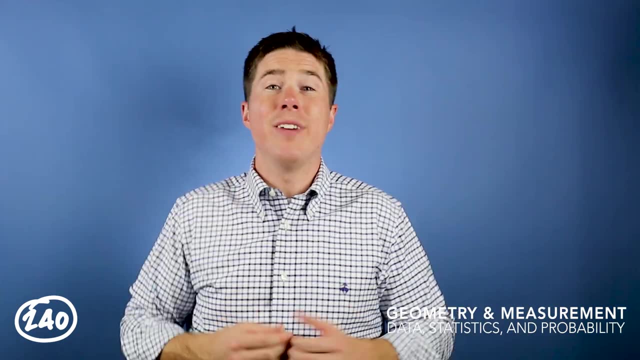 parallel lines, perpendicular lines, angles. Also be able to find the area in the perimeter of two-dimensional shapes, the volume and the surface area of a rectangular prism. Finally, know what the coordinate plane is and how to solve problems with it. 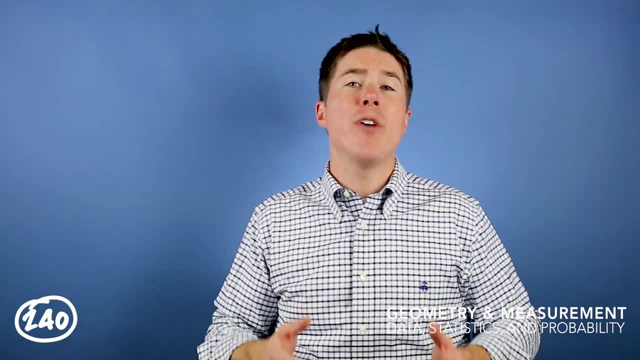 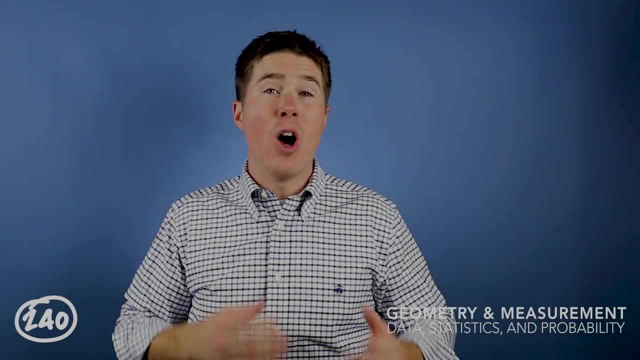 The next big concept to know concerns measurement. Be comfortable solving measurement problems with elapsed time, with money, length and accuracy. The next big concept to know concerns measurement. Be comfortable solving measurement problems with length, volume and mass. Also, you will be asked to measure and compare objects, so be familiar with the customary. 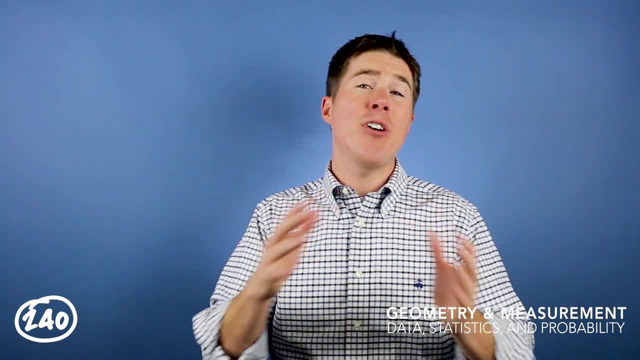 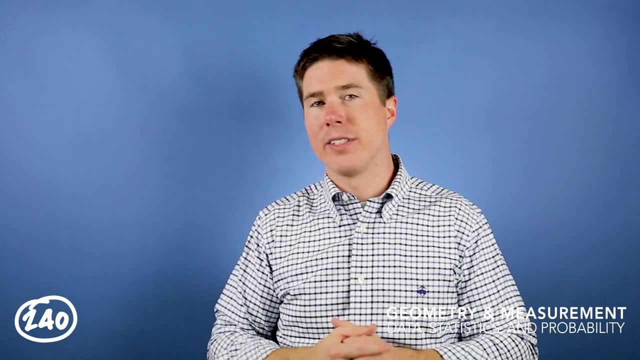 and metric measurement systems. Now again, if all this seems like a lot, it's because it is. There's just so much to know on the exam, and if you want to pass it you have to study. The good news is 240. Tutoring has already done all the hard work. 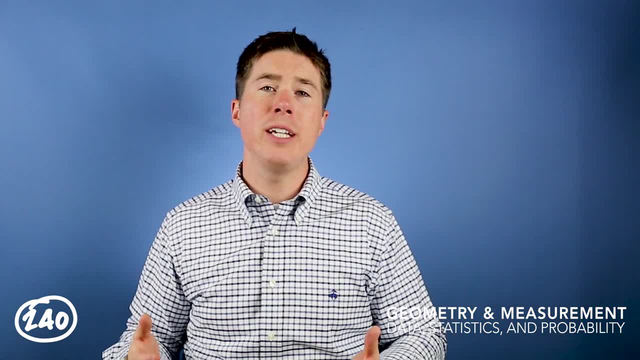 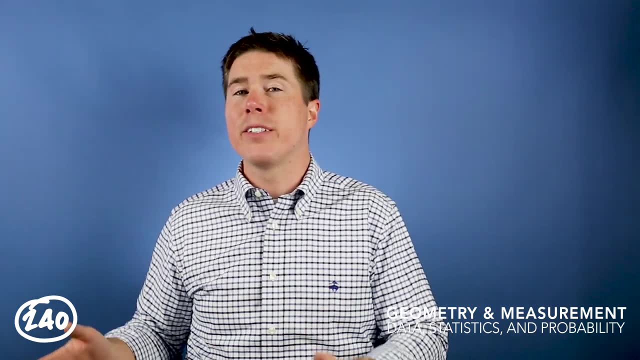 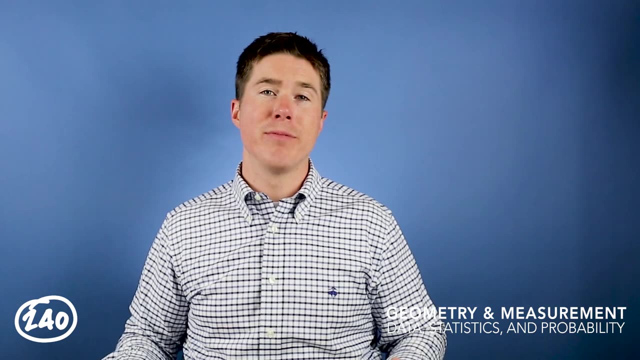 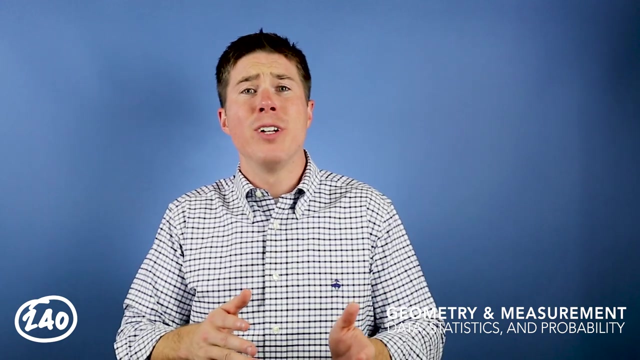 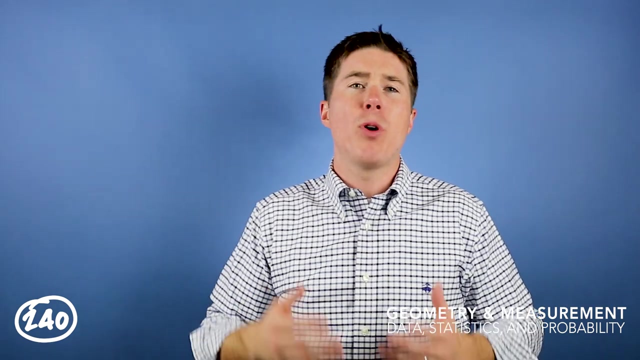 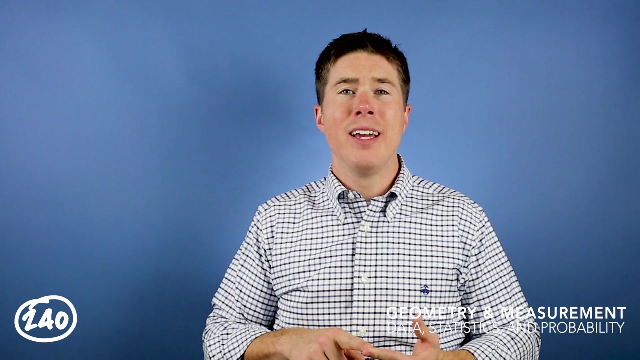 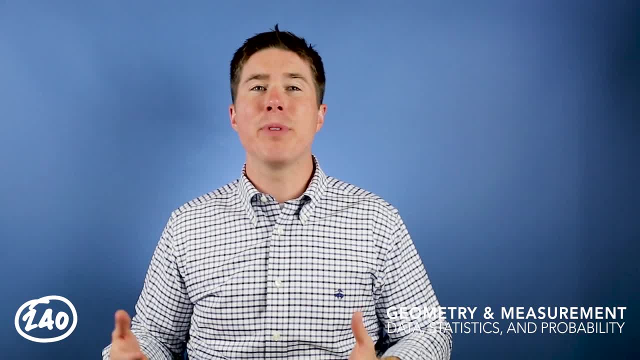 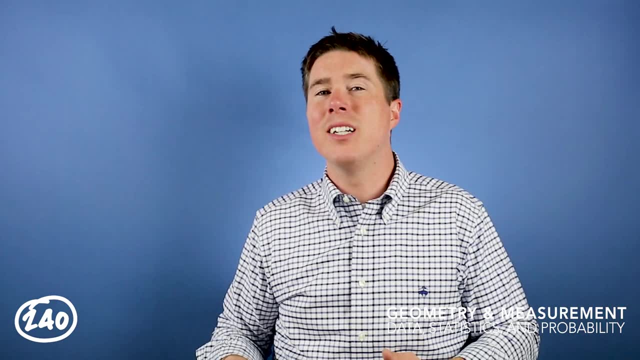 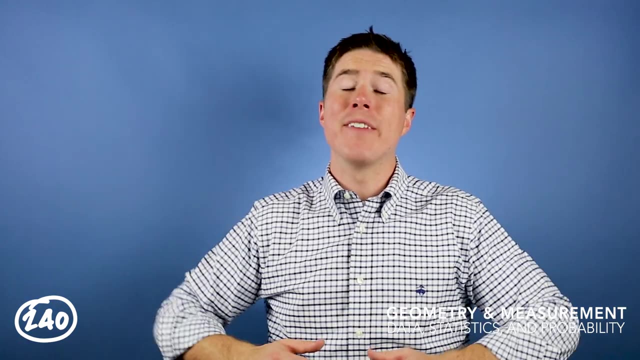 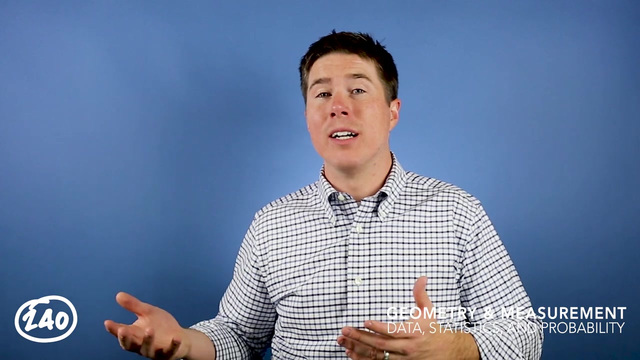 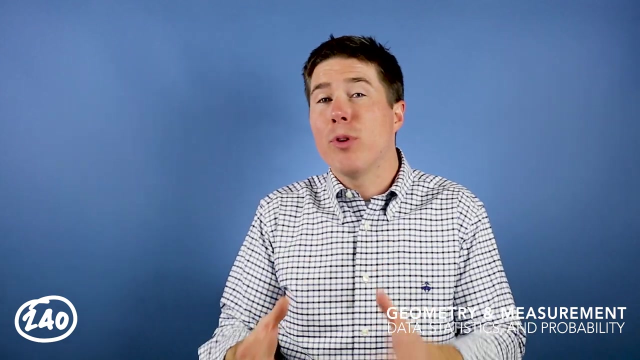 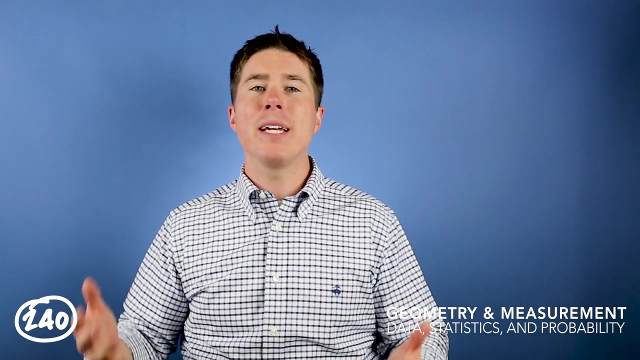 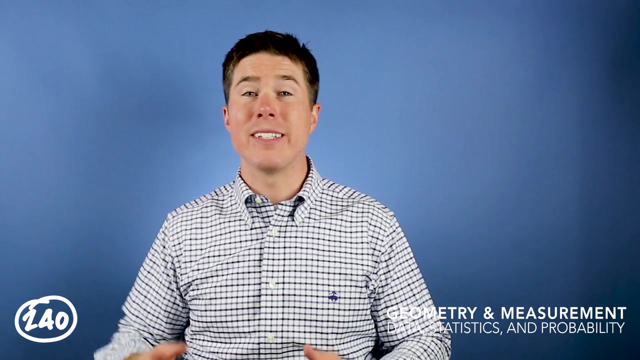 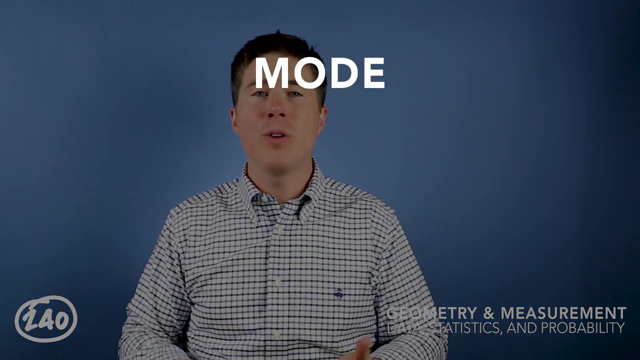 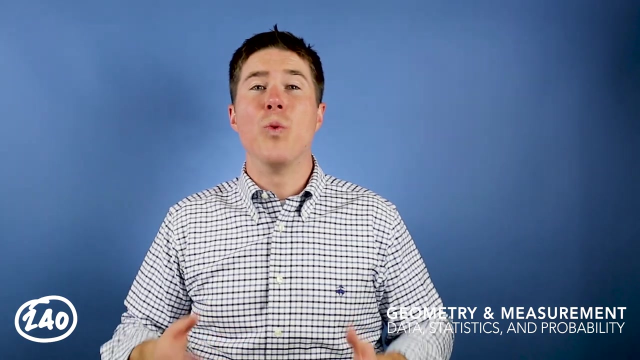 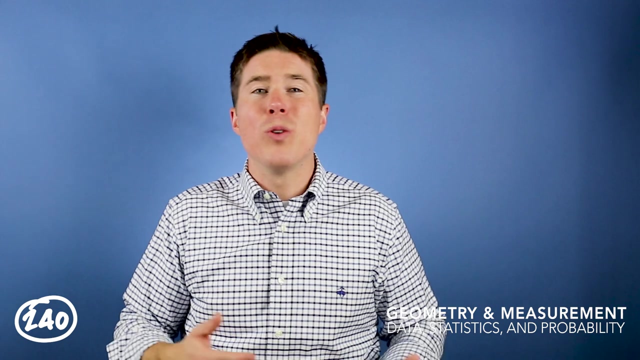 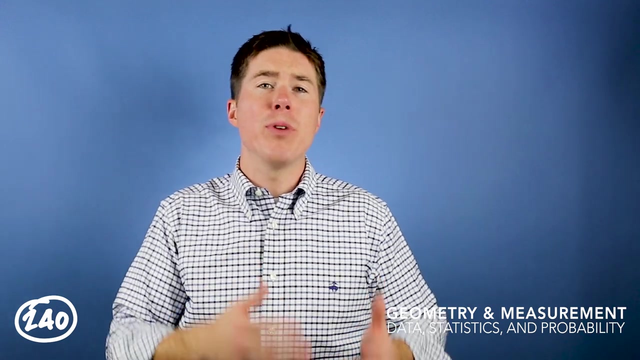 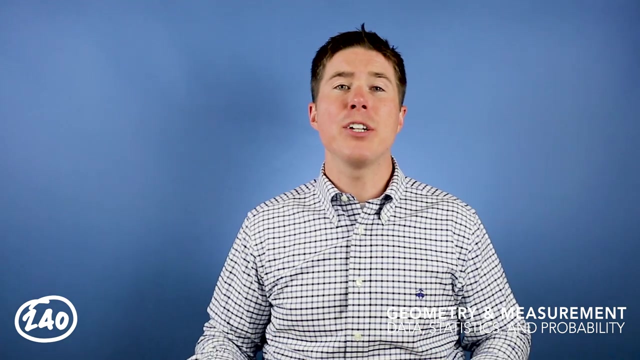 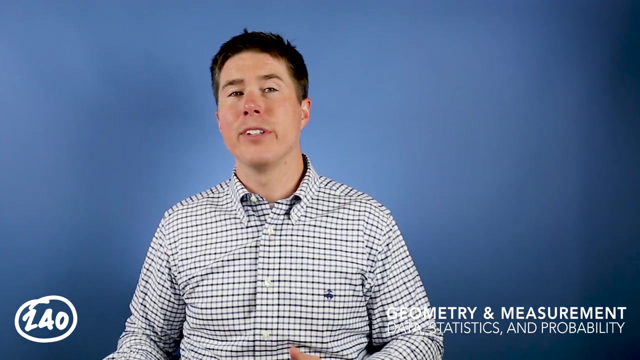 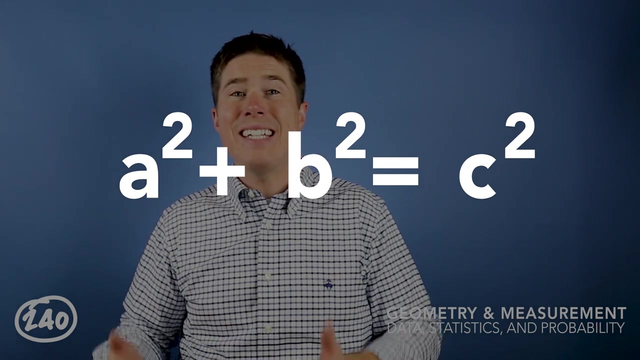 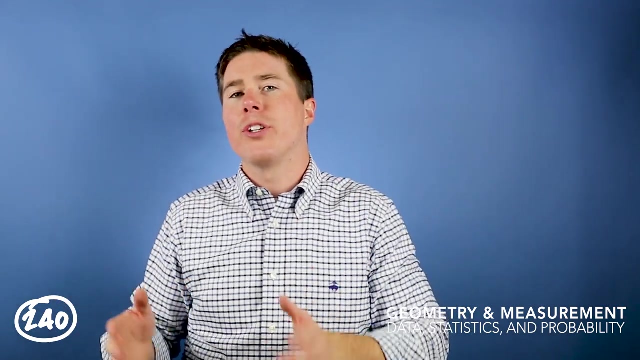 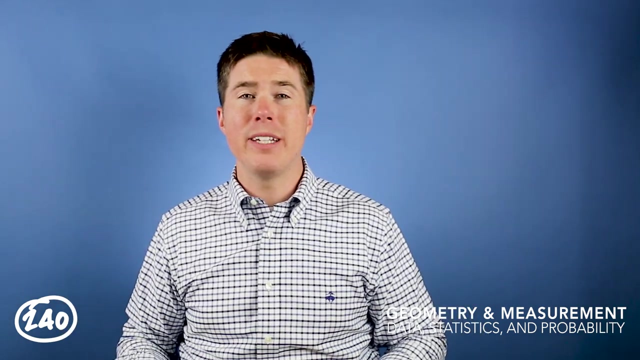 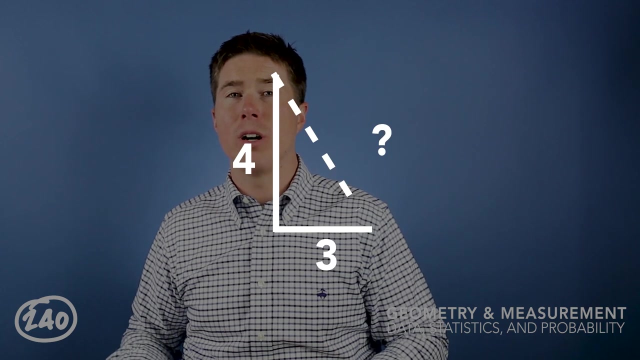 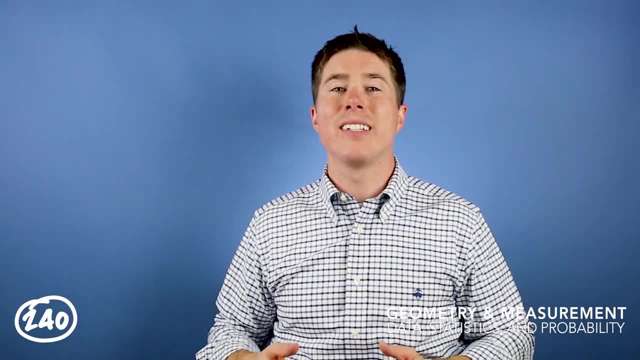 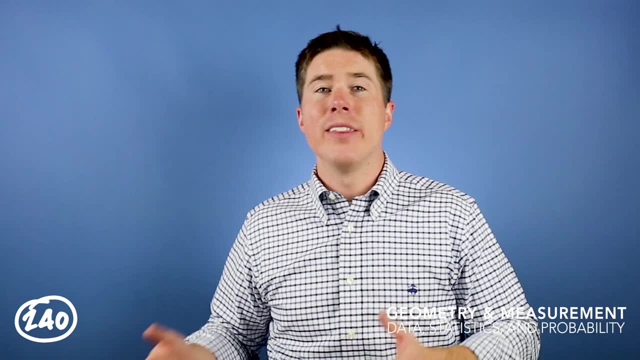 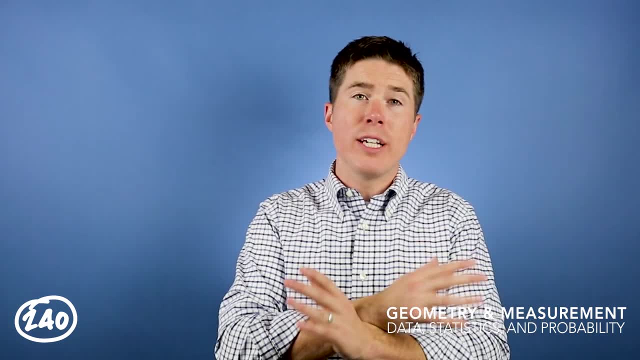 The X-axis is horizontal and the Y-axis is vertical. It has 4 quadrants sections and an origin located at the intersection of the coordinates. You use a coordinate plane to plot points and graph lines and shapes. You use a coordinate plane to plot points and graph lines and shapes. 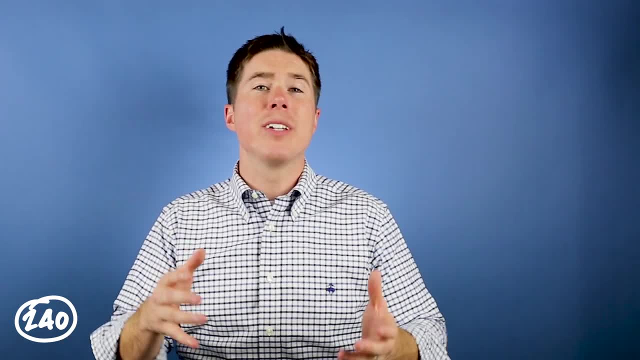 Now, those are the concepts you have to know on the test. so I want to take a few moments and look at a few practice questions in each of those areas and then we can continue to in each of those areas to see how these concepts might actually appear on the test.